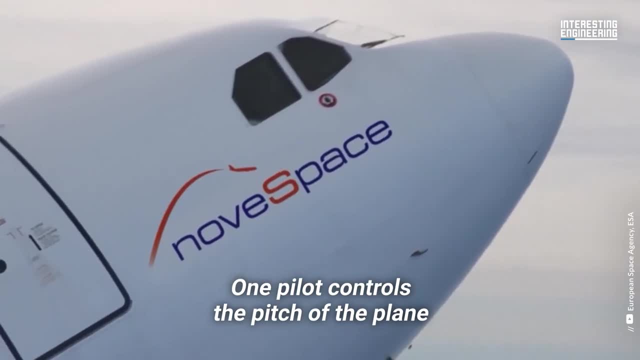 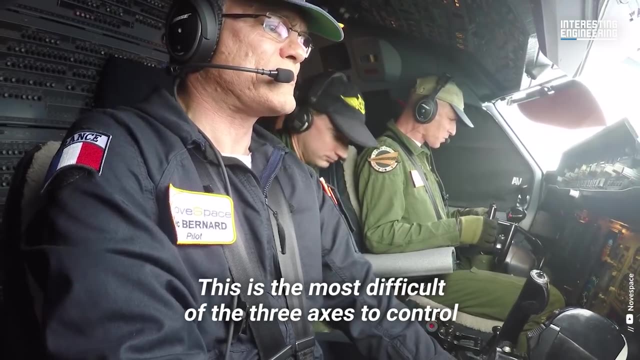 specific axis. One pilot controls the pitch of the plane or the nose-up and nose-down angle. This is the plane that controls the pitch of the plane. This is the most difficult of the three axes to control. A second pilot controls the roll. 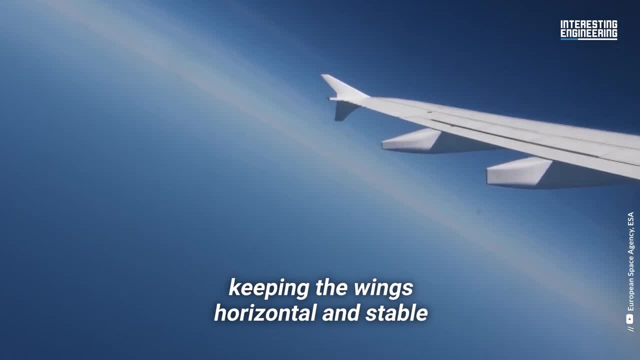 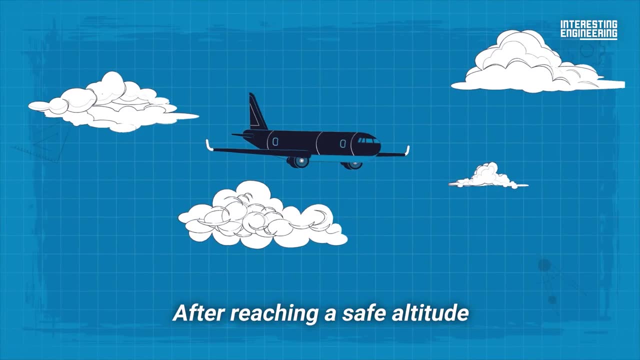 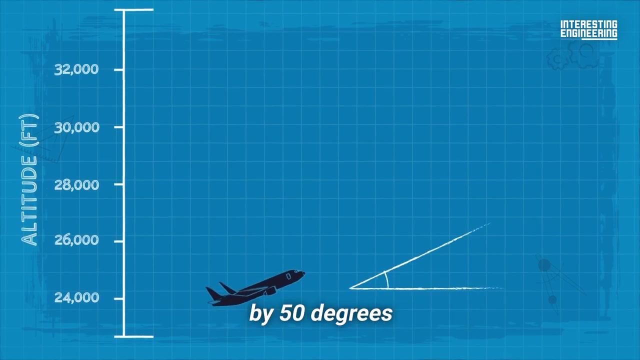 movement, keeping the wings horizontal and stable. The third pilot handles the engine speed and monitors flight parameters. After reaching a safe altitude, one of the pilots starts a sharp climb, lifting the nose of the plane up by 50 degrees. This is the pull-up, the upward approach toward the peak of the parabola. 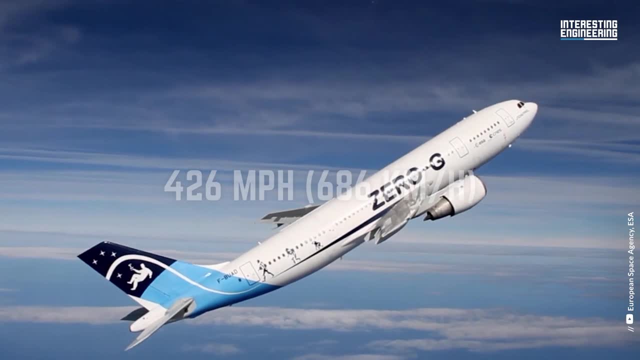 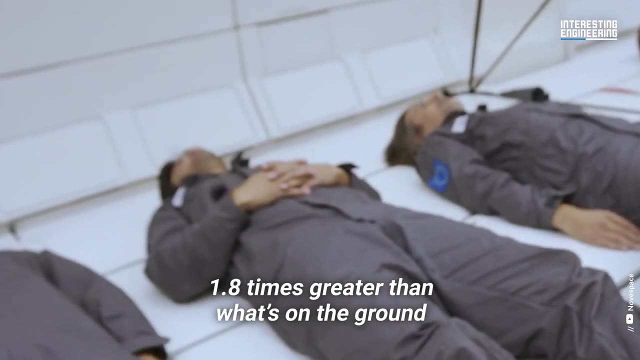 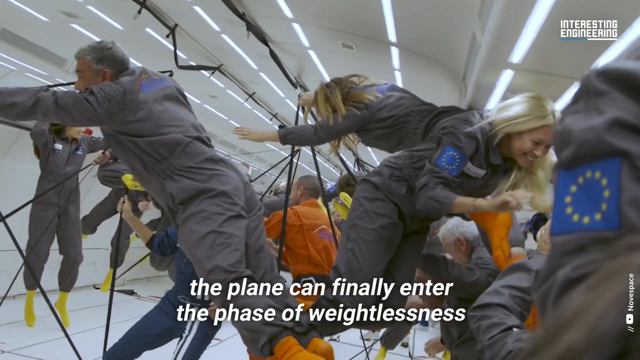 The plane peaks At 426 miles per hour during this maneuver, subjecting everyone on board to a gravitational force 1.8 times greater than what's on the ground for about 20 seconds. Once the pull-up is complete, the plane can finally enter the phase of weightlessness. 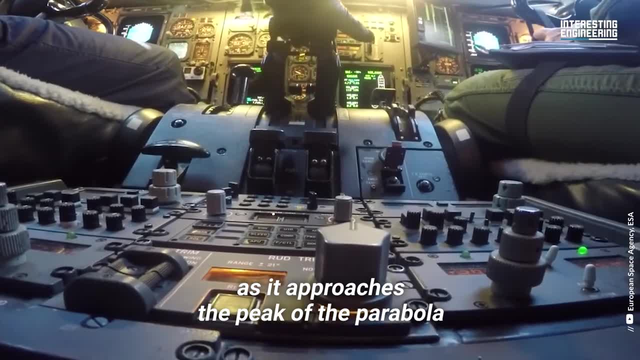 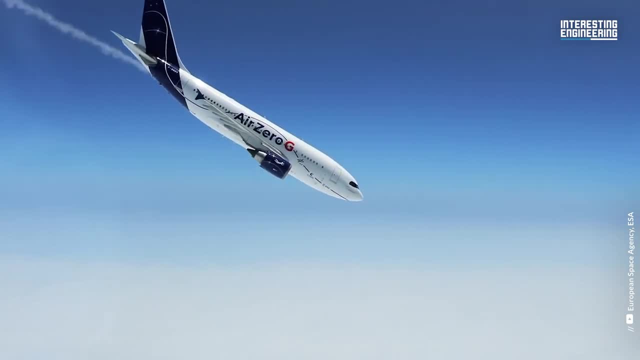 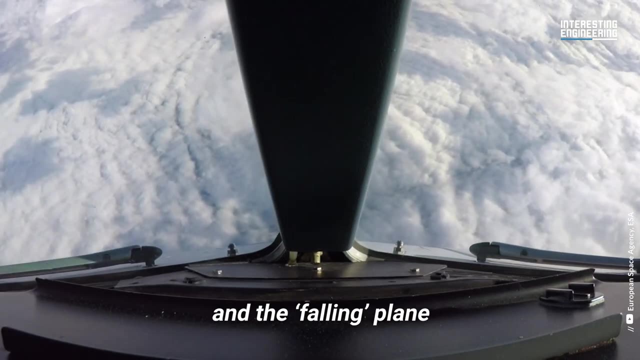 The pilots gradually reduce the plane's engine speed as it approaches the peak of the parabola, and then it free-falls. At this point there's a brief 22-second window where the opposing forces of gravity and the falling plane immediately cancel each other out. Thus there's weightlessness. 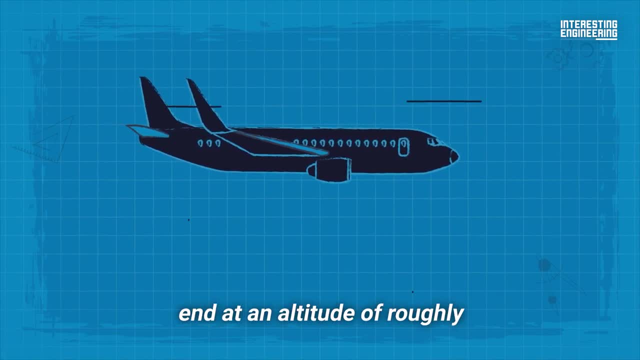 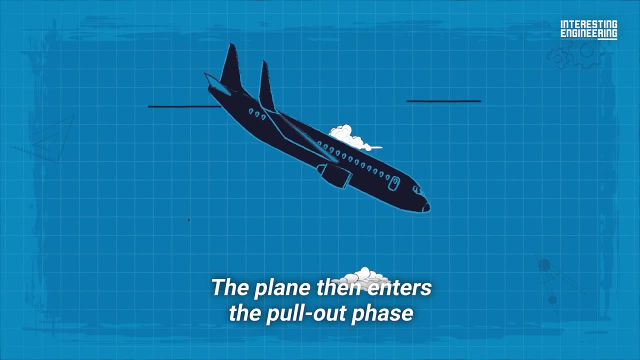 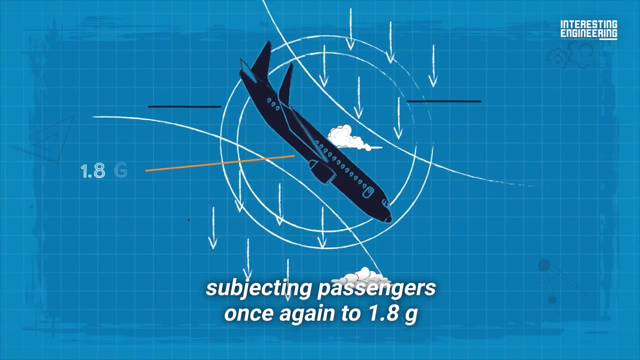 These 22 seconds start and end at an altitude of roughly 25,000 feet, peaking at nearly 28,000 feet in the air. The plane then enters the pull-out phase of its flight path. It accelerates downward, subjecting passengers once again to 1.8 g, before stabilizing to a more. 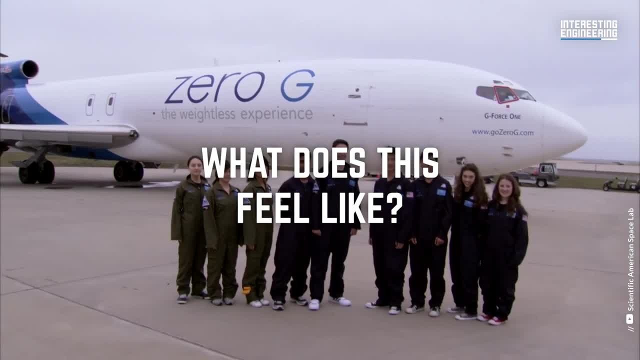 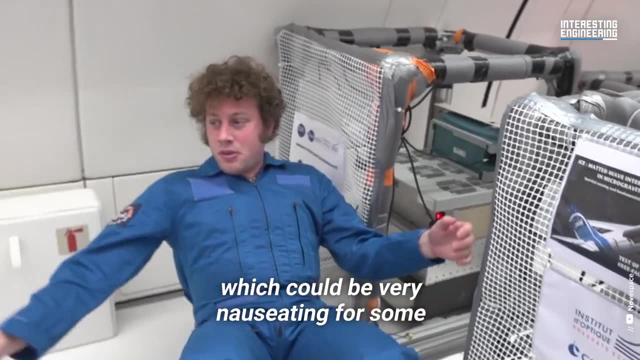 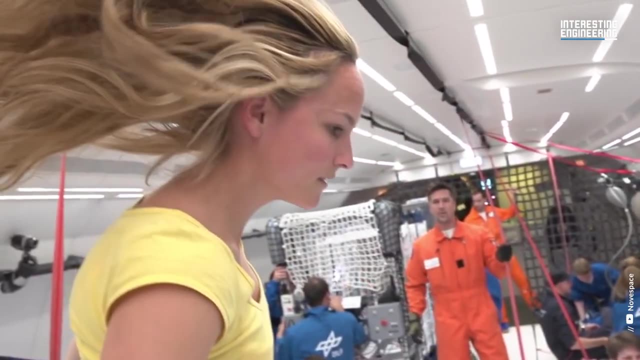 conventional horizontal path. So what does this feel like? The sudden shift can cause blood to rapidly flow to your head, which could be very nauseating for some. This is why zero-gravity planes are also known as the Vomit Comet- Vomit Comet. 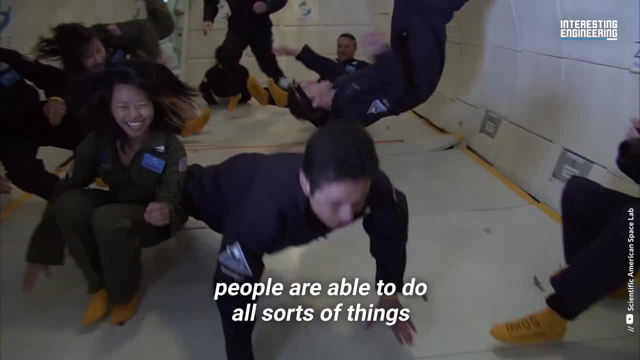 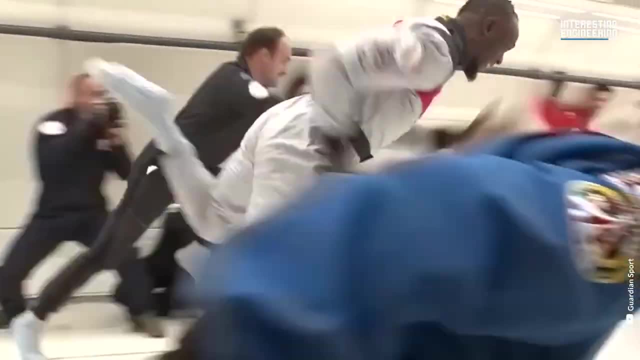 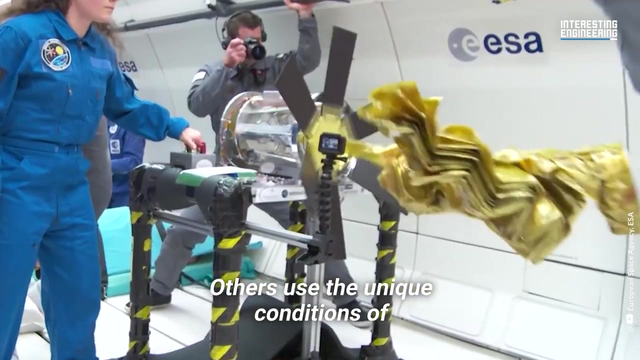 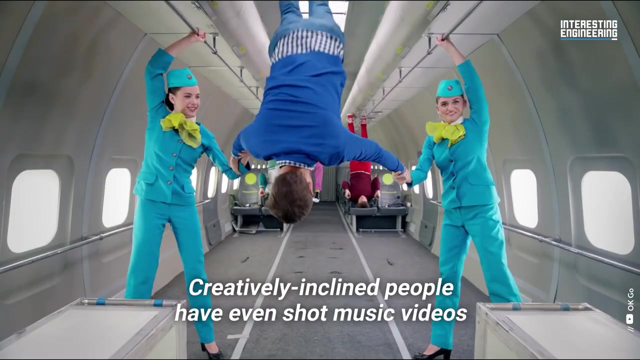 Despite the initial discomfort, people are able to do all sorts of things during zero-gravity flight. Some people board these flights as part of their astronaut training. Others use the unique conditions of zero-gravity flight to perform scientific experiments. creatively inclined people have even shot music videos.